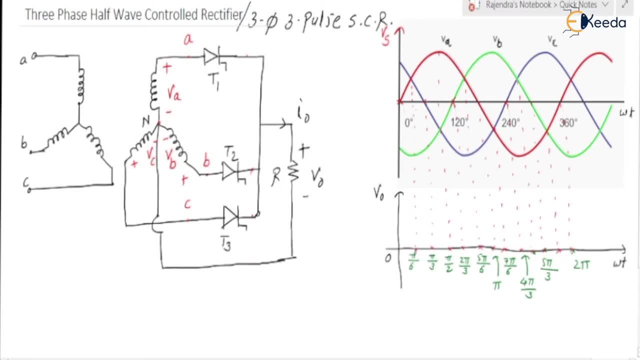 12 sub intervals. right, each interval is of 30 degree. okay, So this is the pi by 6, this is the 2. pi by 6 is nothing but pi by 3,. yes, pi by 2, 2, pi by 3, 5, pi by 6, 6. 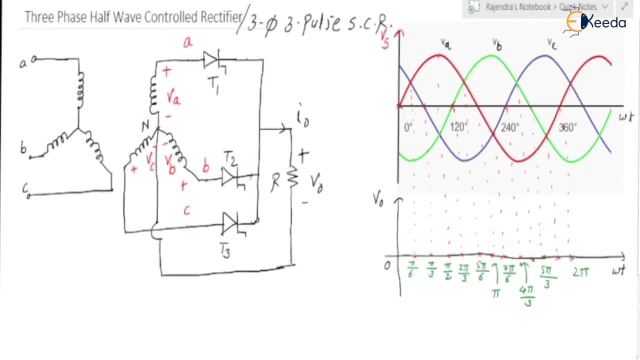 pi by 6, that is the pi 7 pi by 6, here it is the 8 pi by 6,, that is nothing but the pi by 3.. Next, here it is the 5 pi by 3, 11 pi by 6, and here it is 12 pi by 6,. 12 pi by 6 is nothing. 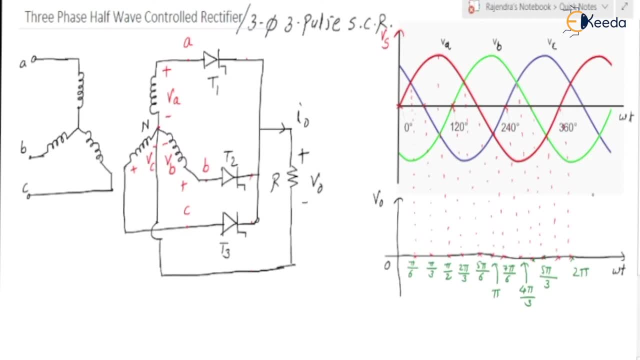 but the 2 pi. okay. So now, in order to initiate, in order to initiate the AC to DC convergence, okay, so here, at omega T is equal to zero degree. at omega T is equal to zero degree. yes, if you check after, omega T is equal to zero, Va is switching into the positive values. 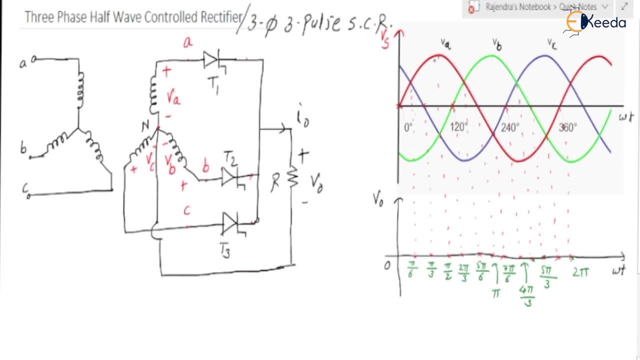 right. So after omega T is equal to zero degree, Va is switching into the positive values, right into the positive values. okay, so, as va is switching into the positive value, so if you check when t1 is in the on state, at that time the output voltage will be equal to va. okay, so i am going to 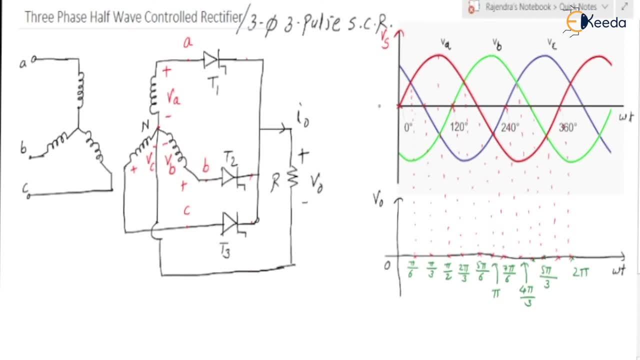 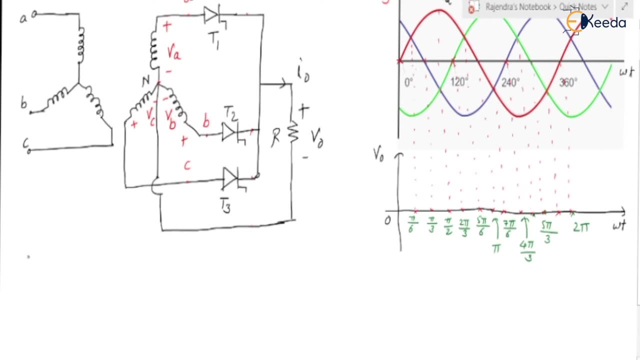 apply the gate pulse to thyristor t1. at omega t is equal to 0 degree. okay, so here: at omega t is equal to 0. i am writing here: at omega t is equal to 0 degree. at omega t is equal to 0 degree. yes. 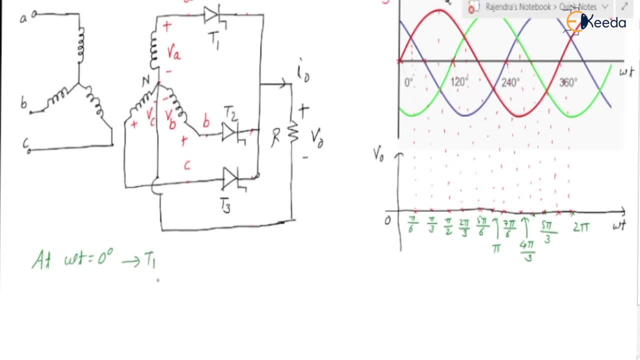 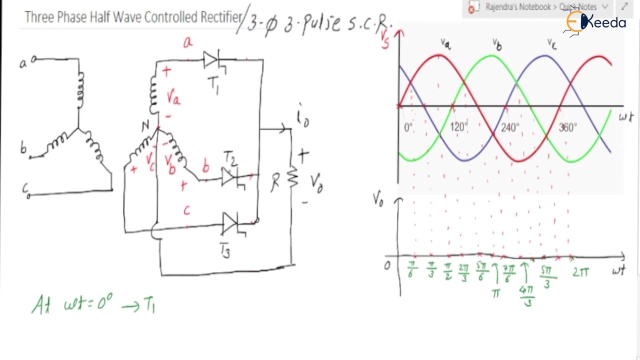 we are going to apply the gate pulse to thyristor t1. okay, similarly, by keeping the same logic. by keeping the same logic, if you check yes, vb, vb is switching into the positive values. vb is switching into the positive values after 120 degree. okay, so if you check yes, when t2 is in the on state at 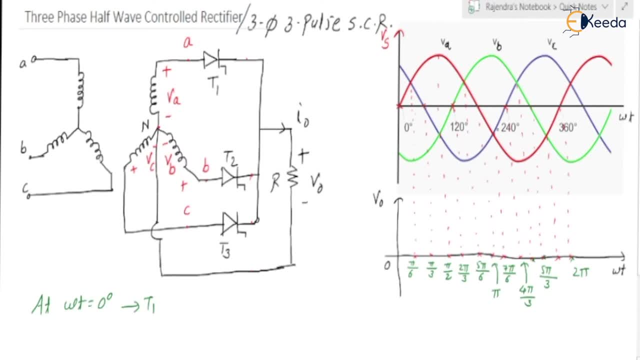 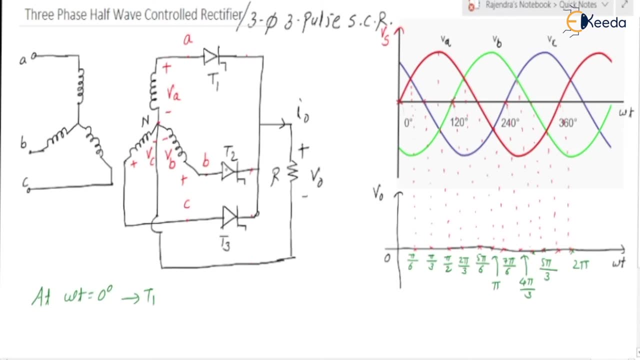 that time vb will appear as an output voltage. okay, so here by in order to keep the same logic: yes, at omega t is equal to 120 degree, we need to apply the gate pulse to thyristor t2, okay. similarly, if you check, vc is switching into the positive values after 240 degree. okay. 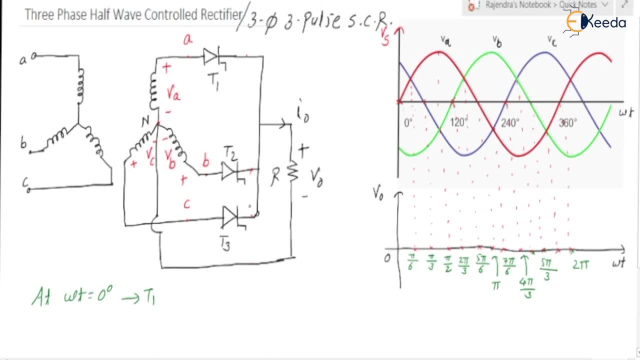 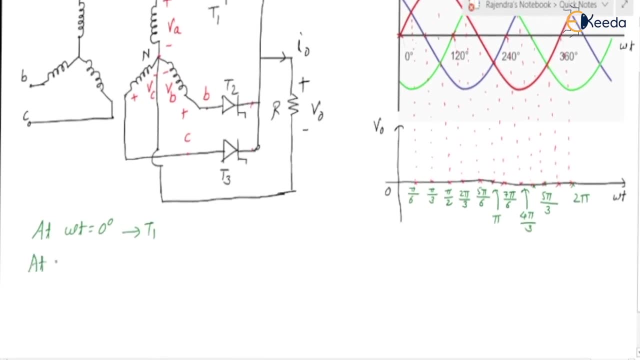 so, at omega t is equal to 240 degree, yes, we need to apply the gate pulse to thyristor t3. okay, so in order to keep the same logic, yes, at omega t is equal to 120 degree, we need to apply the gate pulse to thyristor t2, and at omega t is equal to 240 degree, we need to. 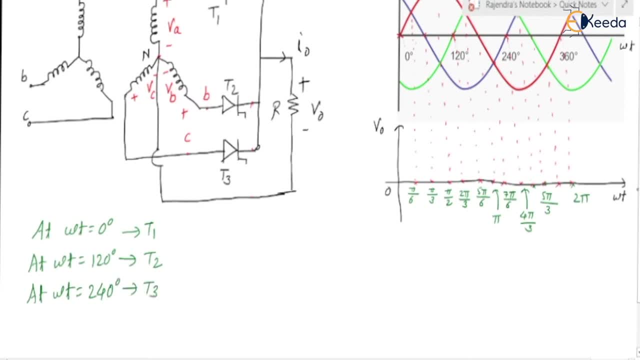 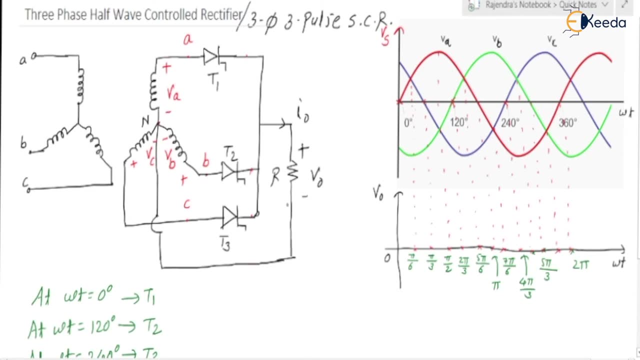 to apply the gate first to thyristor T3,. okay, So here, yes, for the very first cycle. very first cycle means what? Before that cycle, none of the thyristor was in the on state. okay, So at omega. 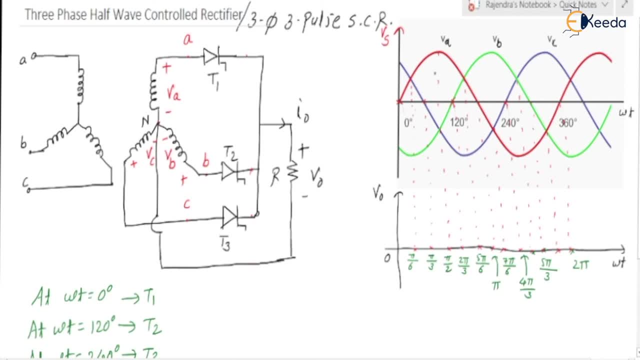 T is equal to 0,. right At omega, T is equal to 0, the thyristor T1 is turned on right. So when thyristor T1 is turned on, it will act as a short circuit. okay, So once T1 turns on, yes, V0 will. 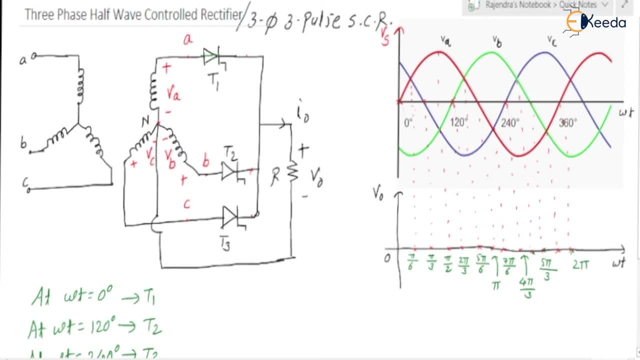 be same as that of the VA right, V0 will be same as that of the VA right. So here this will continue till omega. T is equal to 120 degree, because at 120 degree we are going to apply the. 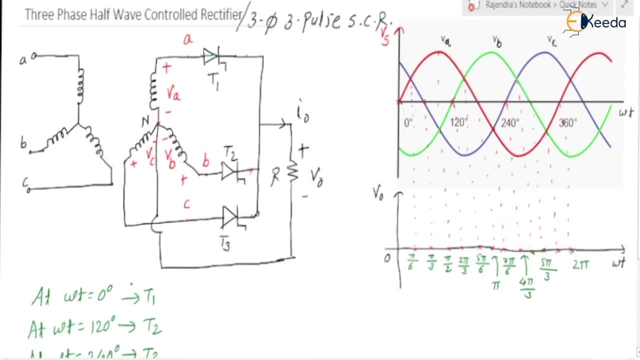 gate signal to the thyristor T2, to the thyristor T2,. okay, So if you check, if the neutral point voltage is 0 volt, then what about the voltage that will be appearing here? This voltage is equal. 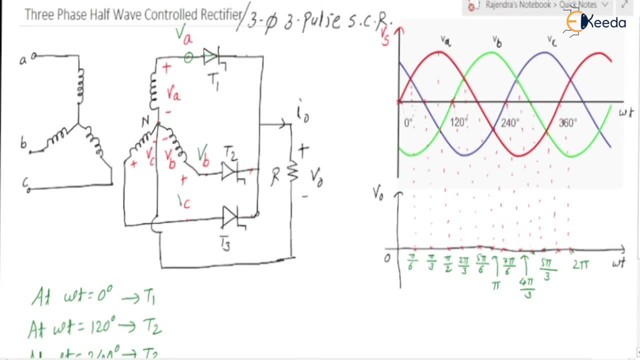 to VA volt, right? This voltage should be equal to VB volt. This voltage should be equal to VC volt. okay, As thyristor T1 is acting as a short circuit, if this is VA, so this voltage is also equal to VA, right? If this is VA, here it is a VA. 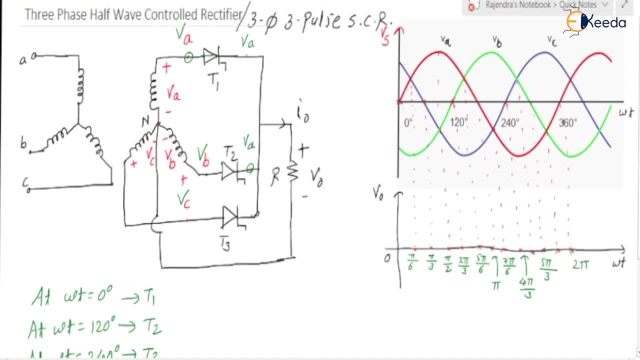 So at the cathode of thyristor T2, the voltage appearing is VA. At the cathode of thyristor T3, the voltage appearing is equal to VA right. So if you check when T1 is in the on state. 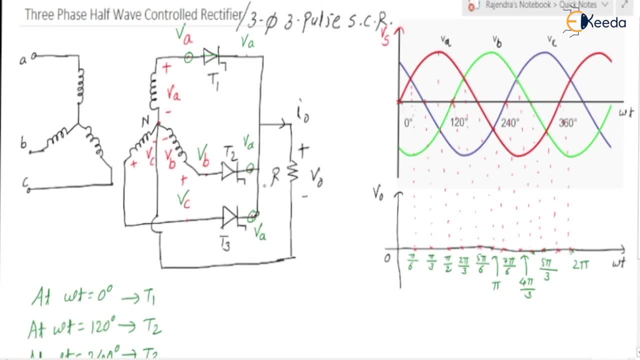 okay, The voltage at the cathode of T2 as well as cathode of T3 is equal to VA volt at the VA volt. okay, So now, after omega, T is equal to 0, when T1 is in the on state, yes, in the output. 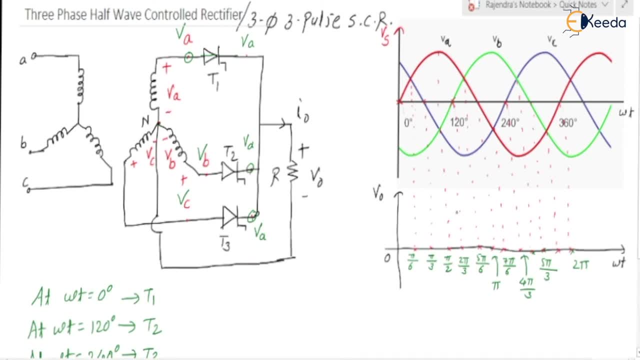 we will be getting the waveform, which is same as that of the VA. okay, This will continue till 120 degree, right? Are you getting the point? okay, So this will continue till 120 degree. 120 is 2 pi by 3, right, It is equal to 2 pi by. okay, So the waveform output voltage. 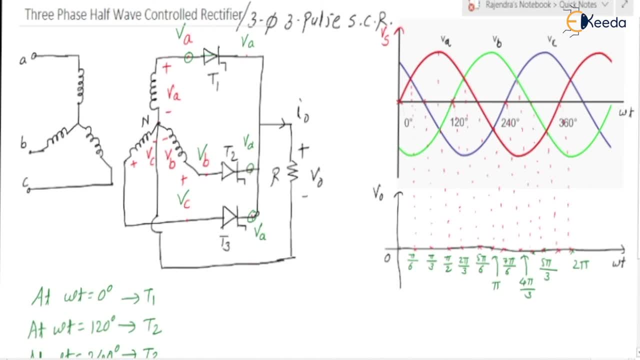 waveform. it will be like this: Whatever the waveform we are having for VA, the same is, yes, same will be copied right As an output voltage for T1, right When T1 is in the on state right. So it is the from here to here. it will be like: 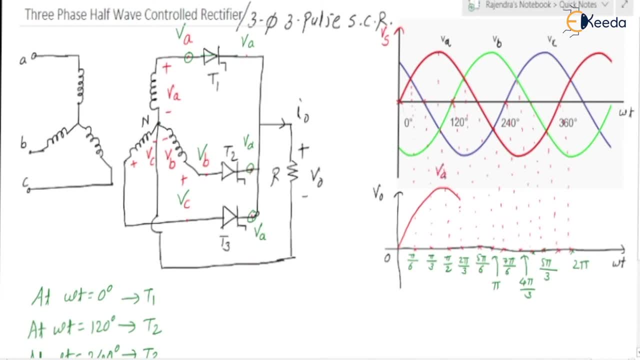 this okay. So this waveform will be same as that of the VA. Are you getting the point, okay? Means from 0 till 2 pi by 3,. our thyristor T1 is in the on state, So that is why output voltage. 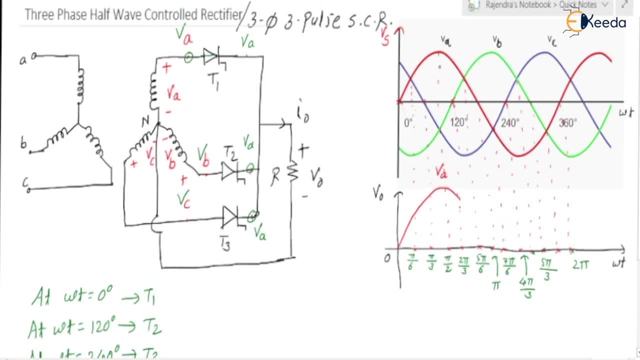 will be same as that of the VA right. So the VA waveform, whatever we are having, the same is repeating here. okay, This will continue till 2 pi by 3.. Again at 2 pi by 3, if you check at 2 pi. 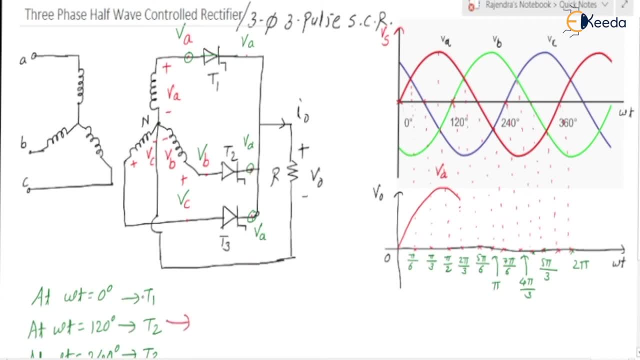 by 3,. we are applying the gate pulse to thyristor T2, okay, So if you check at T2, right Corresponding to omega T is equal to 120 degree. Please check whether thyristor T2 will be in the 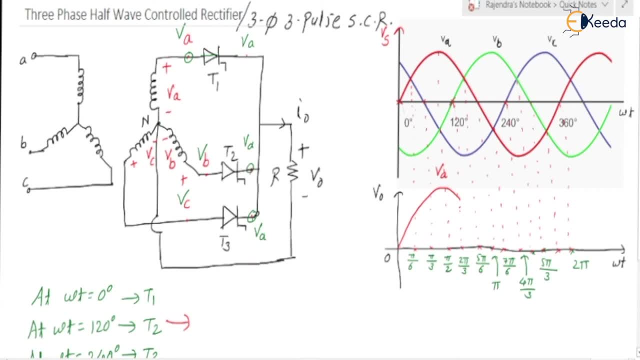 forward bias mode or whether it will be in the reverse bias mode. right, We are applying the gate pulse to T2 at 120 degree, But we need to check whether thyristor T2 is in forward bias mode or whether it is in reverse bias mode at 120 degree. okay, So if you check at 120 degree, 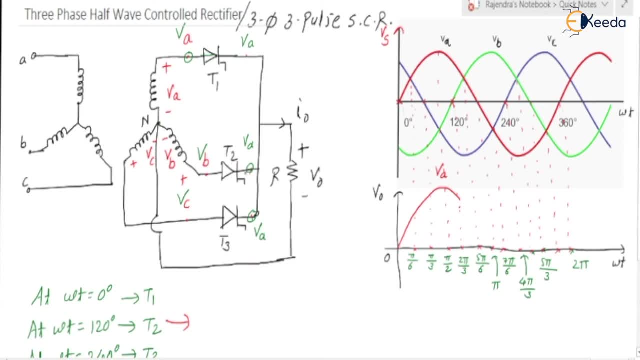 yes, voltage across thyristor T2 is VB minus VA, right? If VB minus VA- it is greater than 0, then thyristor T2 will be in the forward bias mode. okay, So in order to get VB minus VA to be greater than 0, VB should be greater than VA. okay, So if you check at 120, 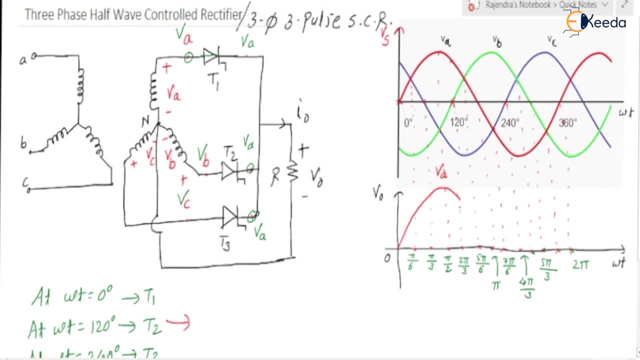 degree. at 120 degree, VB is 0,. VA is positive value. it is a non-zero, okay. So VB is 0 means this voltage is 0, this voltage VA, it is a positive voltage, okay. So whatever the thyristor. 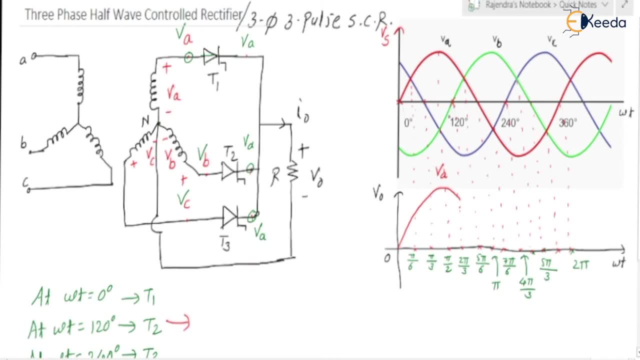 T2 at omega T is equal to 120 degree. yes, at omega T is equal to 120 degree. thyristor T2 will be in reverse bias mode. okay, So thyristor T2 is in reverse bias mode. So whether at omega T is equal. 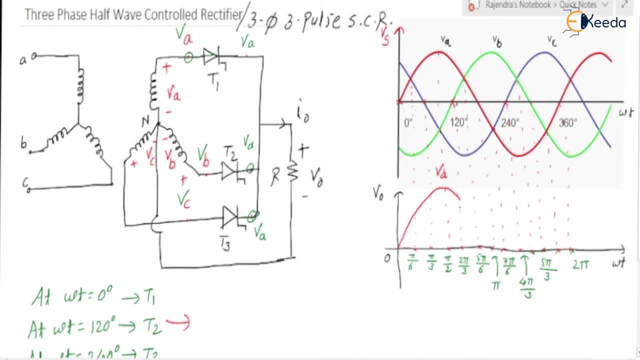 to 120 degree. if we apply the gate signal to thyristor T2, whether our thyristor T2 will turn on? not possible, okay, Thyristor T2 is not turning on. Why? Because at 120 degree thyristor T2 is in. 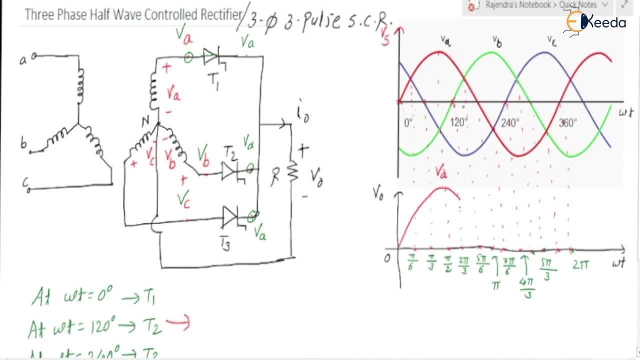 reverse bias mode. Are you getting the point Why the thyristor T2 is in reverse bias mode? Because here, at 120 degree, VB is less than VA, So anode voltage is less than the cathode voltage. So 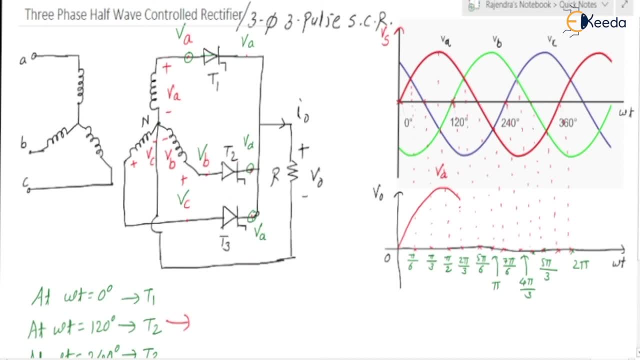 T2 will be in the reverse bias mode. okay, Means, even though if we apply the gate signal at 120 degree right, thyristor T2 will turn on when VB is greater than VA. So, if you check, corresponding to this point, right, corresponding to this point, yes, after this instant, VB is greater than VA. 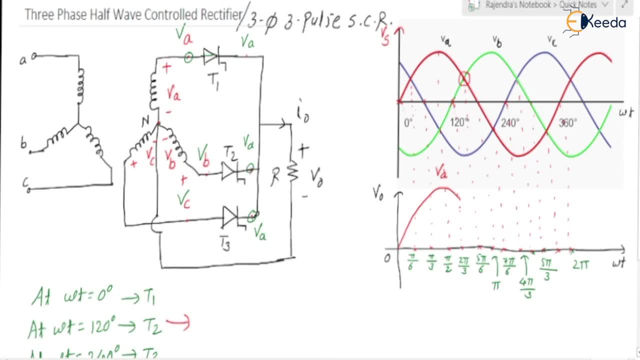 okay, And this point is: it is a 5 pi by 6, right, Are you getting the point? This instant is the 5 pi by 6,. okay, So till 5 pi by 6,. yes, which thyristor will be in the on state? Thyristor T1. 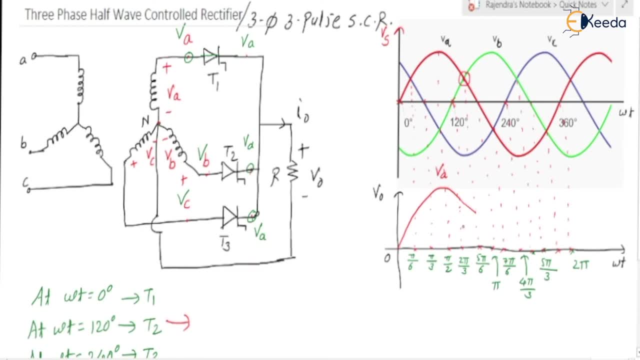 will be in the on state okay. So till 5 pi by 6,. thyristor T1 will be in the on state okay, So it will be only VA okay. Next, at 120 degree, we applied the gate signal to thyristor T2, but T2. 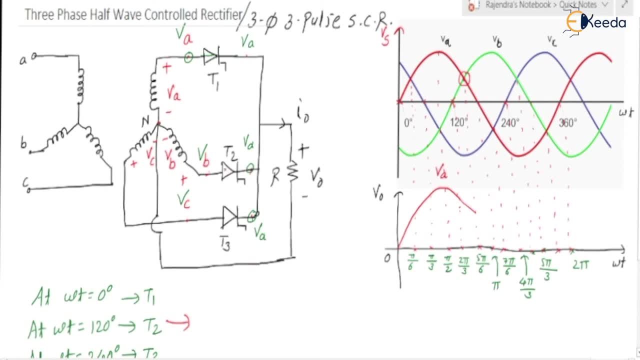 is turning on at 5 pi by 6,. okay, So at 5 pi by 6, at 5 pi by 6, when thyristor T2 turns on, when thyristor T2 turns on, then what will happen to T1? Let us discuss. okay, So at 5 pi by 6,. 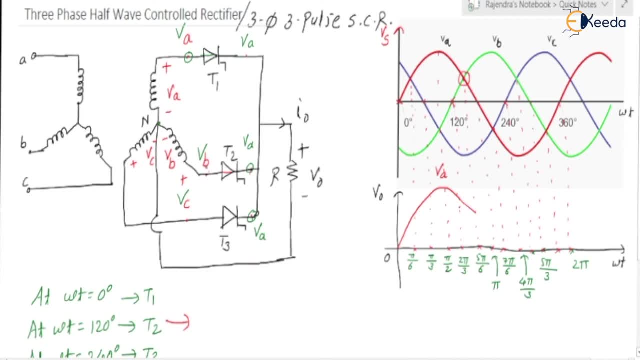 when thyristor T2 turns on. yes, means T2 is acting as a short circuit. So if this here voltage is VB, yes, it is acting as a short circuit. So definitely this voltage should be equal to VB. right, This voltage also should be equal to VB. So if this voltage is acting as a 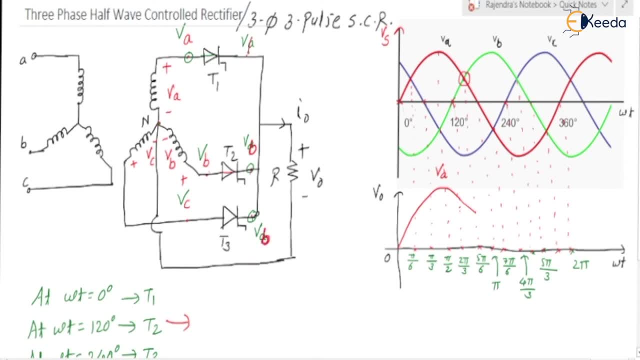 short circuit VB. are you getting the point? okay? And this voltage also should be equal to VB. Is this clear? okay? So after 5 pi by 6, yes, the voltage at the cathode of thyristor T1 and the 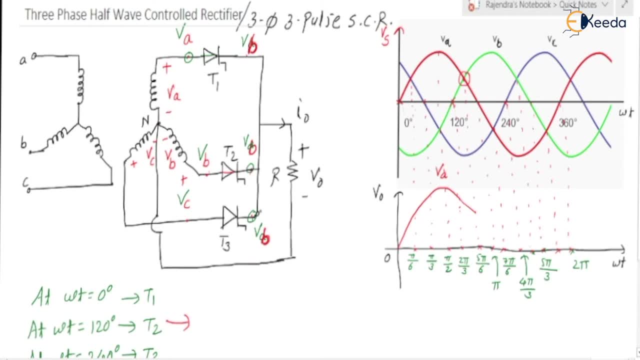 cathode of thyristor T3 is equal to VB volt. that is appearing okay. So if you check T1, okay, after 5 pi by 6, whether thyristor T1 will be in the forward bias mode or whether it will be in. 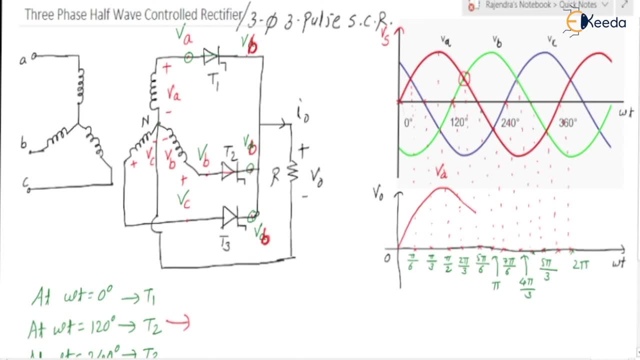 reverse bias mode. okay. So if you check after 5 pi by 6,, yes, VA is less than VB. VA is less than VB means what Anode voltage is less than the cathode voltage. So thyristor T1 will yes. 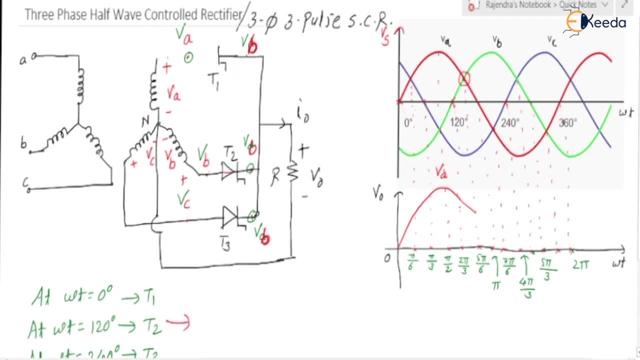 feel the reverse voltage and thyristor T1 will turn off. Are you getting the point, okay? So here thyristor T1 is turning off. thyristor T1 is turning off right at omega. T is equal to 5 pi. 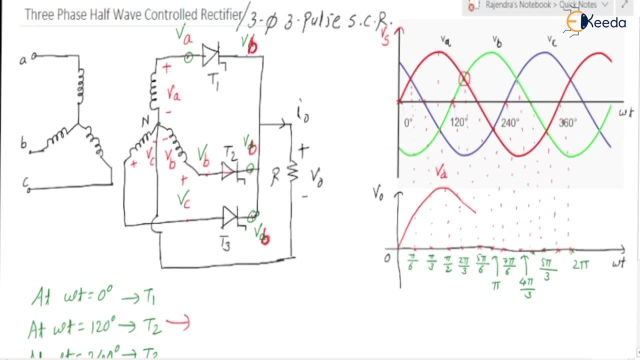 by 6, right At omega T, is equal to 5 pi by 6, thyristor T1 will turn off, okay, So after 5 pi by 6, which thyristor will be in the forward bias mode? Thyristor T1 will turn off, okay, So after. 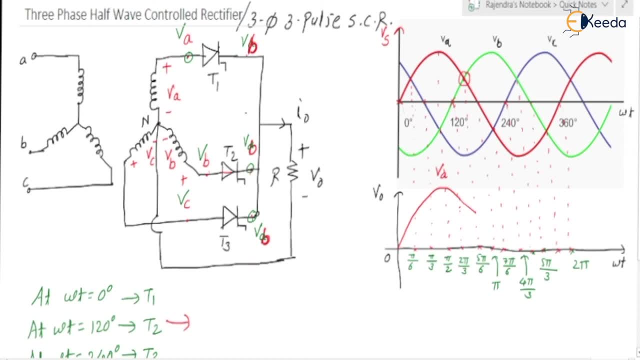 5 pi by 6, till which, till which instant thyristor T2 will be in the on state, Thyristor T2 will be in the on state. till we apply the gate signal to thyristor T3,. right, So we are applying the gate. 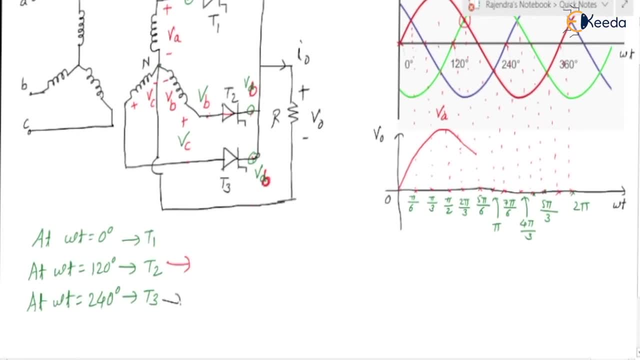 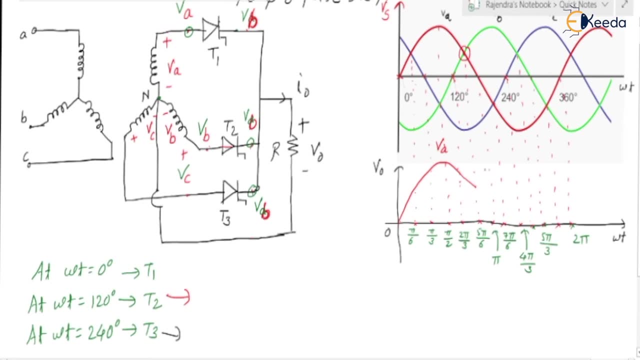 signal to thyristor T3 at, yes, 240 degree. okay, So here, if you check at 240 degree, we are applying the gate signal. okay, So from 5 pi by 6 till 240 degree, our thyristor T2 will. 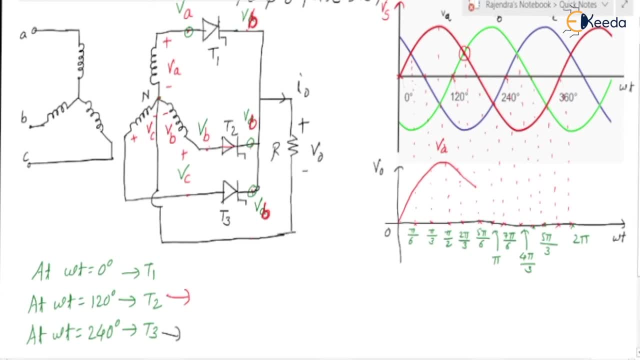 will be in the on state. So when T2 is in the on state, in the output we will be getting VB. okay. So here in the output we will be getting VB right till 240 degree. okay, So it is till. 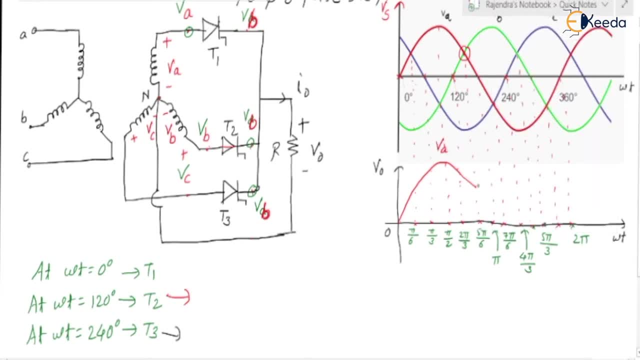 240 degree, right. 240 means this instant, okay. Okay, in the output it is a VB till 240 degree. okay, So at 240 degree. at 240 degree, we are applying the gate pulse to thyristor T3, okay. 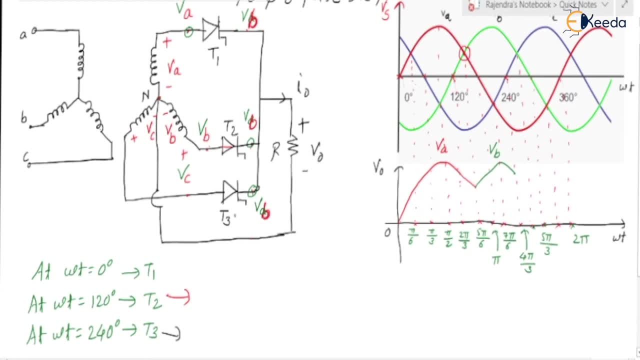 But please check at 240, whether thyristor T3 is in forward bias mode or whether it is in reverse bias mode. So at 240 degree, if you check, the voltage at the anode of thyristor T3 is VC at the cathode of thyristor T3. 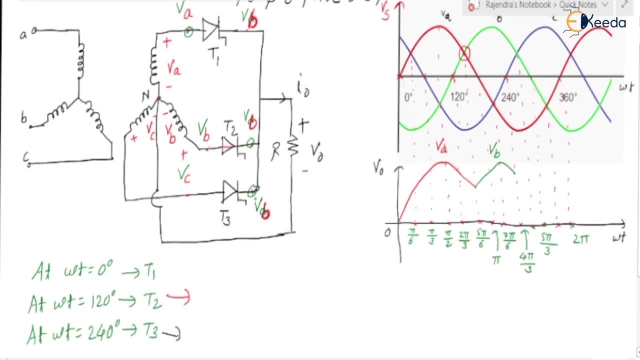 is VB, okay, So please check whether VC is greater than VB or less than VB. okay, So at 240 degree VC is 0, VB is positive. right, So VB positive, VC 0 means thyristor T3 will be in the reverse. 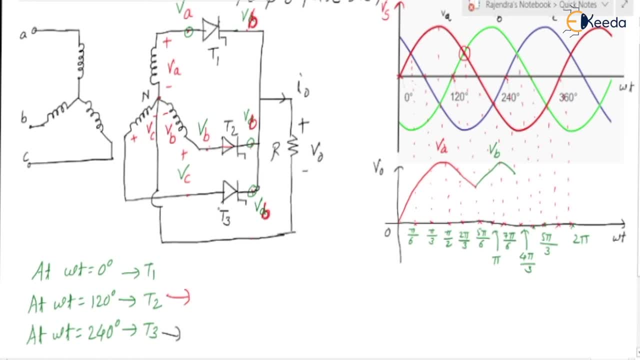 bias mode. okay, So thyristor T3 is in reverse bias mode at omega T is equal to 240 degree. So whether thyristor T3 will turn on? No right, Thyristor T3 will turn on when we apply. yes, when. 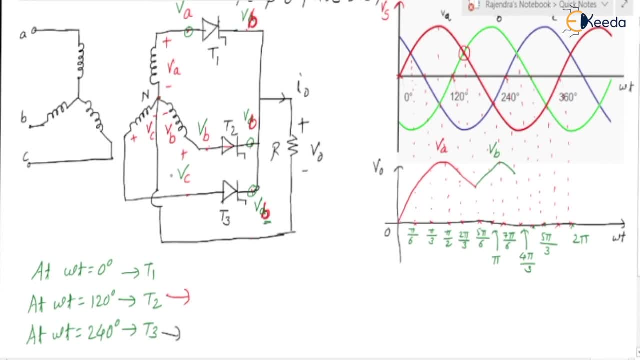 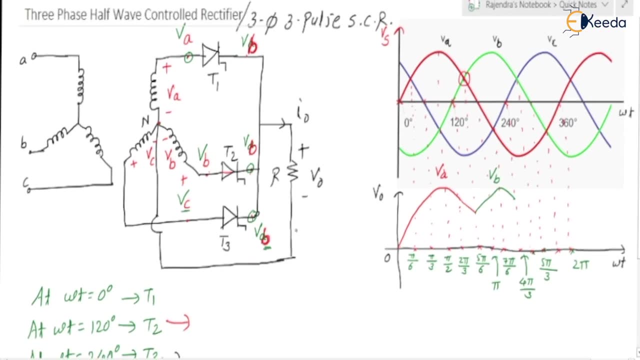 yes, VB becomes greater than VC, right? When VB becomes greater than VC, then, and only then, our thyristor T3 will turn on. okay? So if you check at which instant VB becomes less than VC, right, Thyristor T3 will turn on. when VC becomes greater than VB, okay. So if you check at this instant, 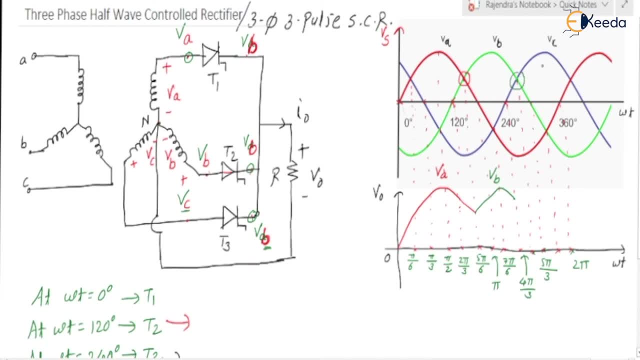 at this instant or after this instant. after this instant, VC is greater than VB, vc is greater than vb. okay, and this instant is nothing. but yes, it is a like. this is 240 degree, right, 240 degree is like. it is a 4 pi by 3. okay, so it is. this is 5 pi by 3. okay, so 7 pi by 6, 8 pi. 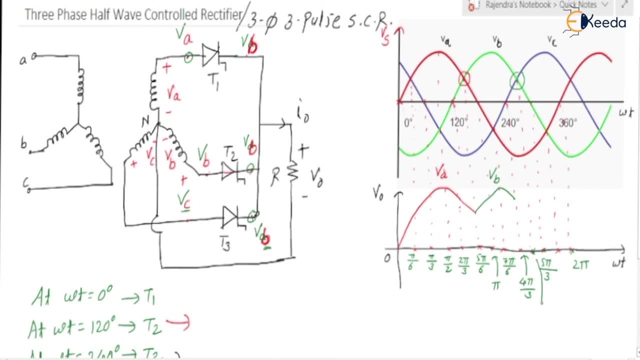 by 6, this is a 9 pi by 6. okay, this is clear. this instant is like a 9 pi by 6, 9 pi by okay. so till 9 pi by 6, our thyristor t2 will be in the on state. okay, so when thyristor t2 is in the on state, 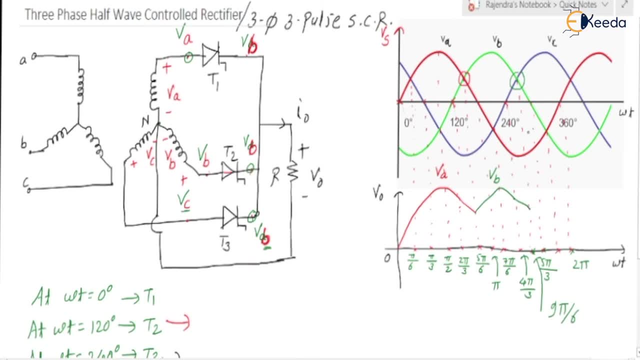 in the output, we will be getting the vb. okay, and after this instant, that is, after 9 pi by 6, after 9 pi by 6, yes, the thyristor t3 will turn on. okay, so thyristor t3 will turn on okay. so once thyristor. 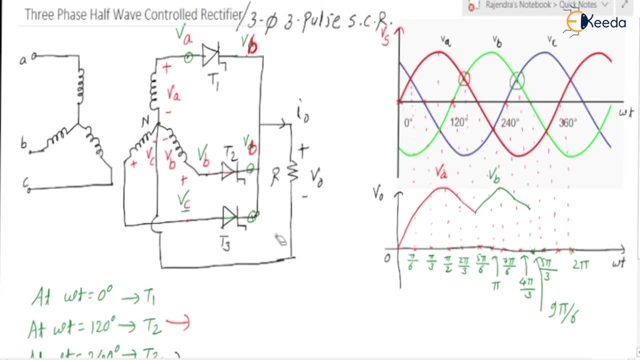 t3 turns on. once thyristor t3 turns on, yes, in the output we will be getting vc right in the output. we will be getting vc okay, so, as thyristor t3 has turned on. so therefore the hair voltage is vc right. so, similarly, if you check, similarly, if we 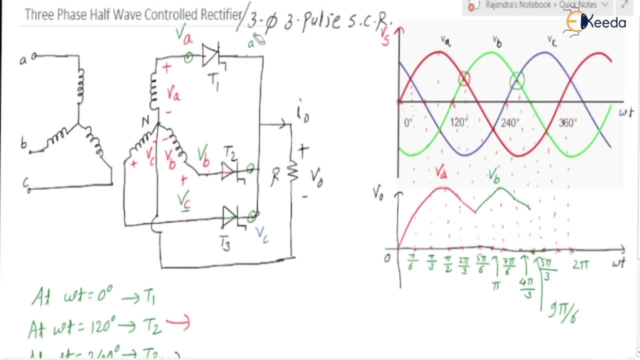 check. yes, voltage that will be appearing at voltage that will be appearing at cathode of t2 as well as cathode of t1 is equal to vc volt. okay, so if you check here, when t3 turns on, what will happen to t2? yes, when t3 turns on, what will happen to t2? yes, check the voltage: vb minus vc. okay, or vb. 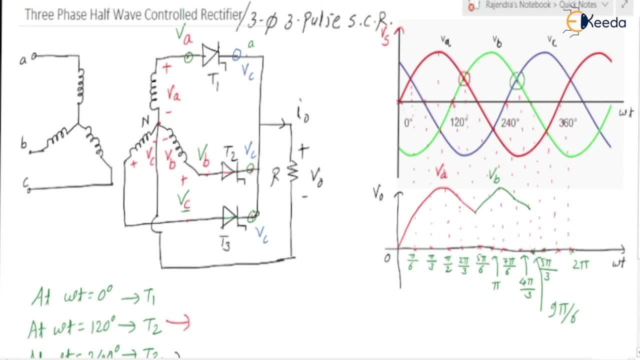 is greater than vc or whether it is a less than vc when t3 turns on. okay. so at this instant t3 is turning on. okay. so if you check after this instant vb is less than vc. so vb less than vc means what thyristor t2 will turn off: thyristor t2 will turn off. are you getting the point okay? 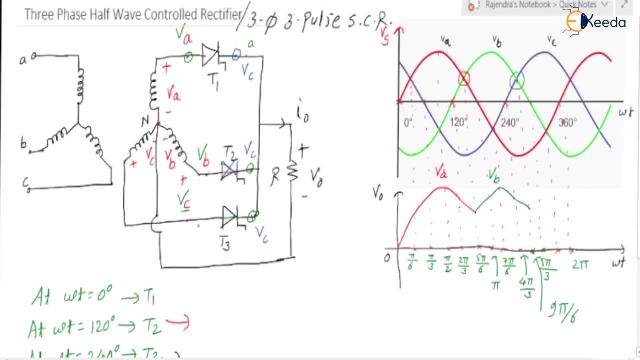 so when t3 turns on, t2 will turn off. okay, so after that in the output we'll be getting only vc waveform. in the output will be getting only vc waveform. right, this will continue till: yes. this will continue till. we apply the gate signal to the yes thyristor t1. we apply the gate signal to the thyristor t1. okay, 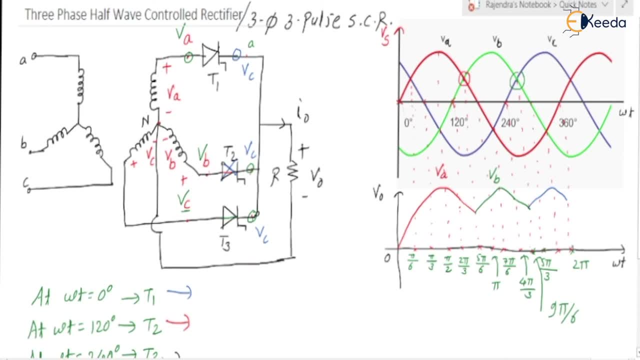 at very first cycle, we applied at 0 degree, right? so therefore, in the continuous cycle, we are supposed to apply gate signal at 360 degree. okay, because after 360 degree, yes, va is switching out into the positive values, right, va is switching into the positive values, okay. so if you check, 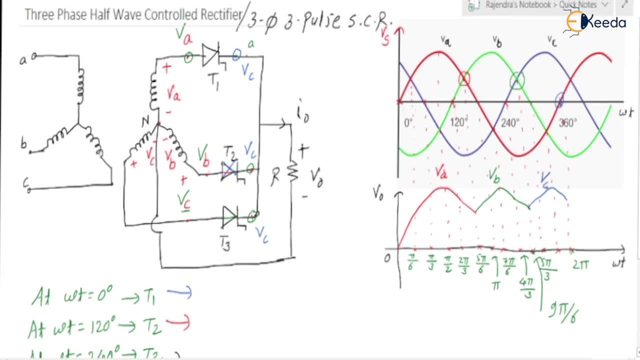 at 360 degree, at 360 degree, right at 360 degree, whether thyristor t1 is in a forward bias mode or whether it is in a reverse bias mode. yes, if you check before 360 degree, thyristor t3 was in the on state, so voltage that was appearing across the thyristor t1 was here. it is a va. 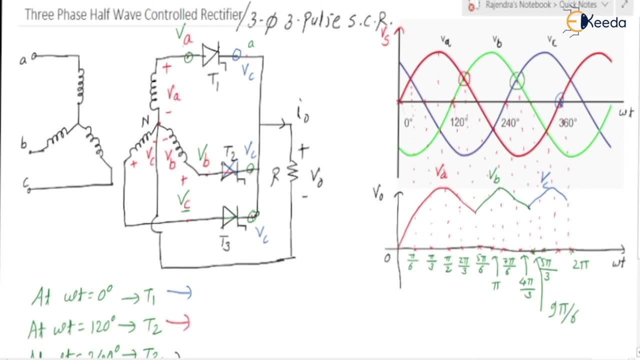 and here it is a vc. okay, so please check at 360 degree. 360 degree is nothing but again zero degree, right? because one complete cycle, yes or no, 360 degree, is again equal to zero degree. okay, so please check at zero degree. yes, whether va is greater than vc or less than vc, yes, va is zero. 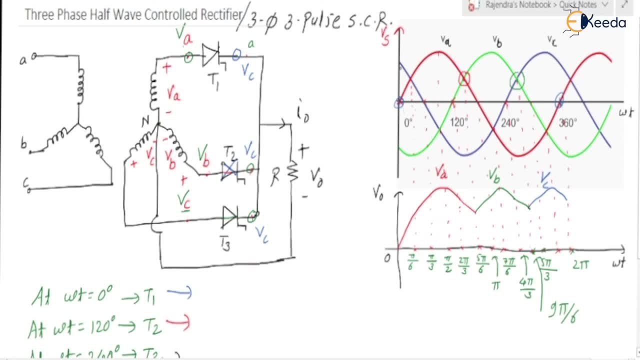 and here it is. vc means the blue curve. okay, so vc is greater than va, right? so if vc is greater than vm is thyristor t1 will be in the reverse bias mode. okay means even though if we apply the gate pulse to thyristor t1 at zero degree in continuous cycle, i am saying okay for very. 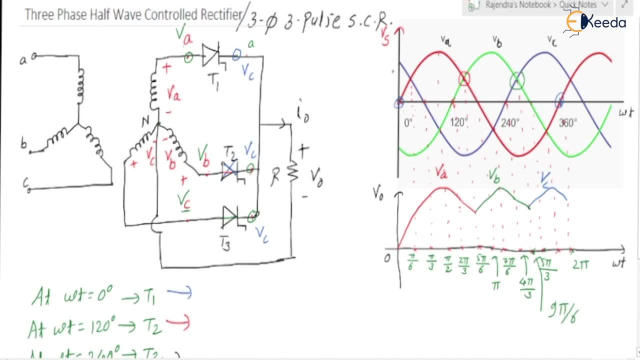 first cycle? definitely it will turn on. okay, but at for continuous cycle. if we apply the gate signal to thyristor t1 at zero degree, okay, then what will happen? whether our thyristor t1 will turn on, no, thyristor t1 will turn on at pipe, at. 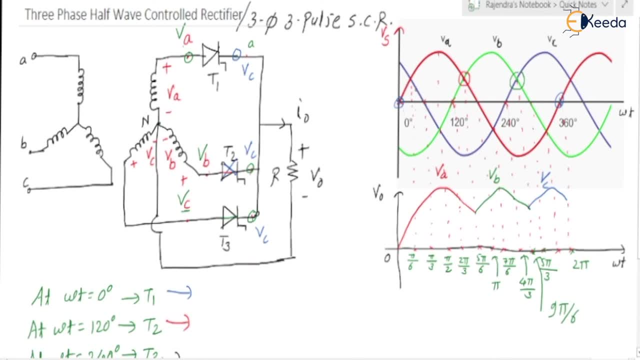 pi by six. when the, when va becomes greater than vc, right, when va becomes greater than vc, then, and only then, our thyristor t1 will turn on. okay, so till that instant, till till that instant, which was the thyristor t3, so when t3 is in the on state in the output will be getting vc waveform in the. 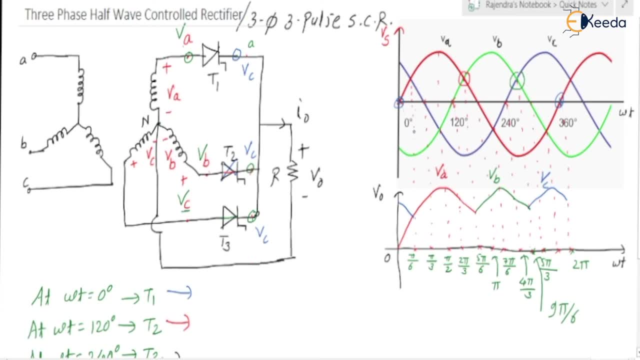 output will be getting vc waveform. okay. so here, if you check, for very first cycle, va will start from zero. okay, but for continuous cycle. but for continuous cycle it will be, but for continuous cycle it will be starting from. it will be starting from pi by six only. it will be starting from pi by 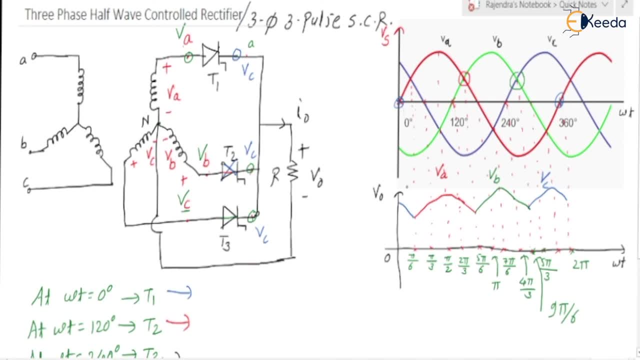 six only, okay. so if you check the output will be getting the waveform like this: okay, this is the sum part of the vc. after that, from pi vi, six till the next instant, we'll be getting the va right, that is, pi by six to five, pi by six va. okay. next we'll be getting vb in the output from five, pi by six till. 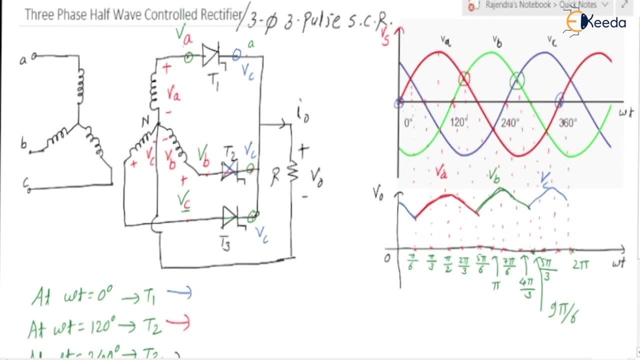 nine pi by six. okay, so it is from five pi by six till by 6 and 5 pi by 6 till 9 pi by 6. it is same as that of the vb, okay, and after that we will be getting the vc from 9 pi by 6 till this instant. okay, so it is a vc. okay. so here can we say that. 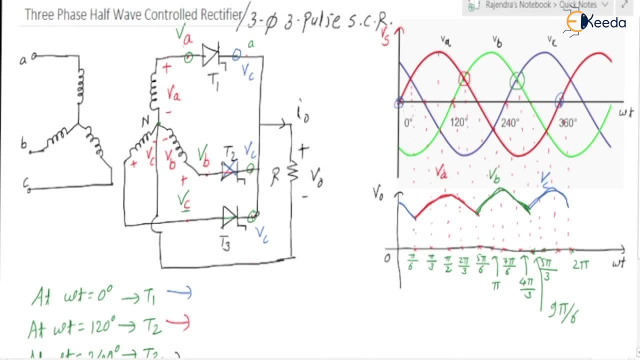 from pi by 6 to 5 pi by 6. yes, thyristor, t1 is in the on state. yes, from here to here, t1 is in the on state. okay, next, from this point to this point: yes, t2 will be in the on state. 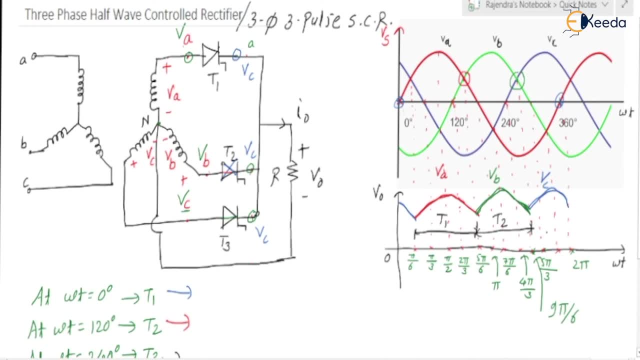 yes, t2 will be in the on state here and here after this instant. yes, t3 on state here also. t3 here also. we are having the t3 in the on state is clear. okay, so if you check, each thyristor conducts for 120 degree. okay, it is from 5 pi by 6 to 5 pi by 6, so it is a 120 degree. 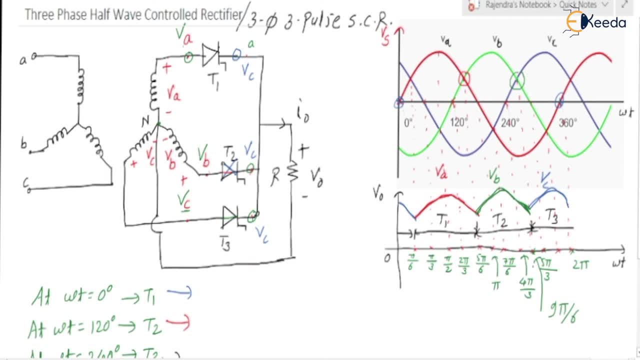 let's see here, second thyristor: 5 pi by 6 to 9 pi by 6.. So again it is a 120 degree, right, And it is a 9 pi by 6 till again next 2 pi plus pi by 6, okay, So that is again 120 degree, okay. So next, if you check, 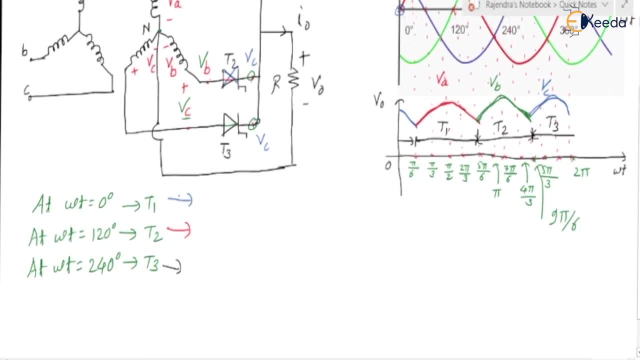 yes, we have developed a logic that at omega, t is equal to 0 degree. we are going to apply the gate signal to thyristor T1, okay, But for the continuous cycle, at what instant thyristor T1 will turn on? At pi by 6, actually, okay, So thyristor T1 will not turn on at 0 degree, okay. 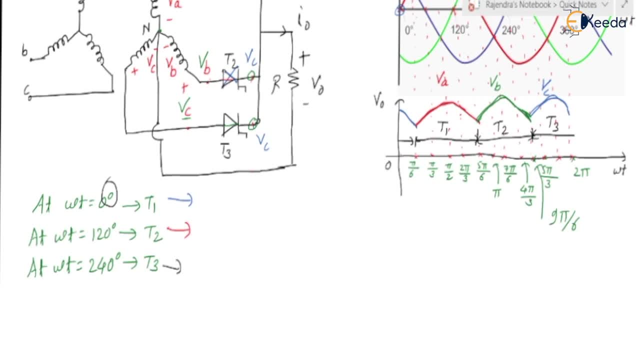 So thyristor T1 will not turn on at 0 degree, right, But it will turn on at pi by 6.. It will turn on at pi by 6,. okay, It will turn on at pi by 6,. 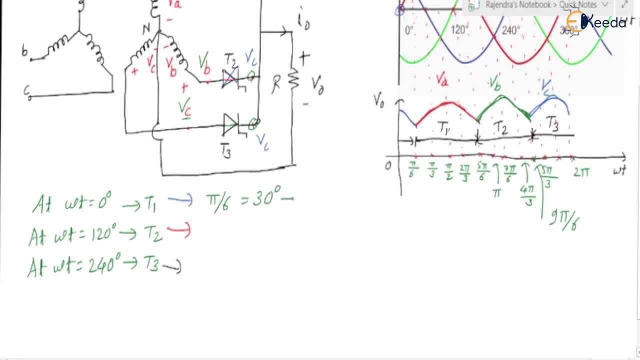 which is equal to 30. Are you getting the point? At 30 degree, thyristor T1 will turn on okay. Next, what about the thyristor T2?? We are applying the gate signal at 120 degree, But actually thyristor T2 will turn on at 5 pi by. 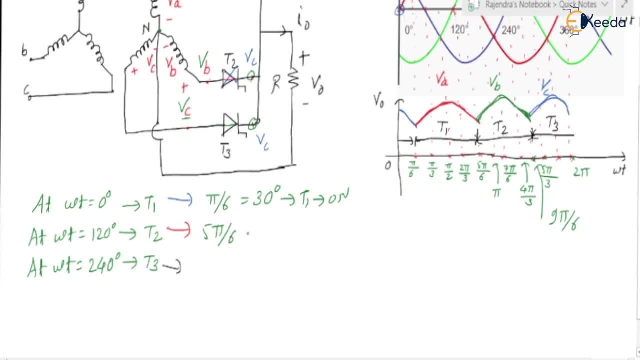 6, right. At 5 pi by 6, thyristor T2 will turn on. Thyristor T2 will turn on right. 5 pi by 6 means what It is equal to 150 degree right. Similarly, at 240 degree, we are applying the gate pulse to. 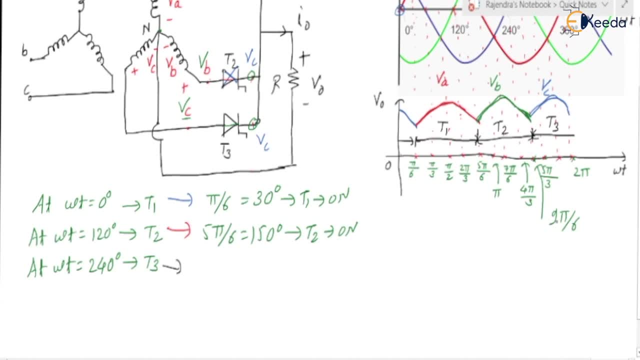 thyristor T3,. right, But thyristor T3 will be turning on at 9 pi by 6,. okay, So it is a 9 pi by 6.. 9 pi by 6, which is equal to what 270 degree right Here thyristor T3 will turn on. Is this clear, Okay? 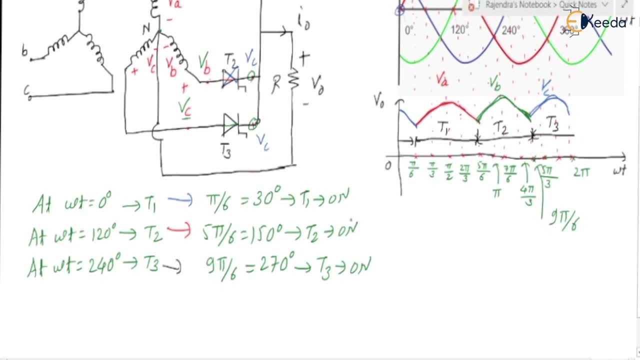 So, if you check right, So thyristor T1 is turning on. Thyristor T1 is turning on at pi by 6, okay, At pi by 6, okay. And if we apply the gate pulse before pi by 6 to thyristor T1, whether thyristor T1 will turn on. 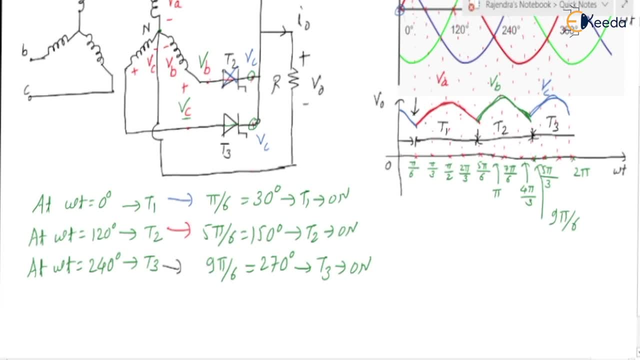 No, because before pi by 6, thyristor T1, yes will be in the reverse bias mode. okay, So can we say that this is nothing but alpha equal to 0 degree for thyristor T1, right? Similarly. 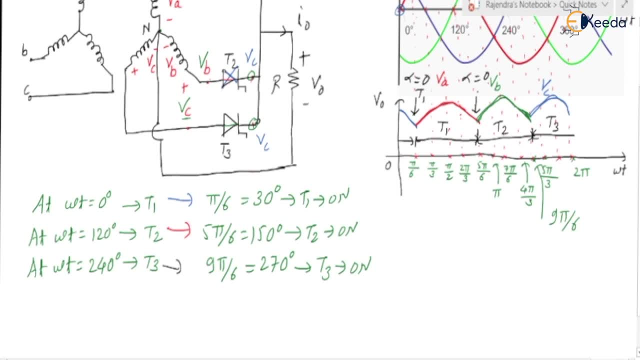 this is nothing but alpha equal to 0 degree for thyristor T2. and this is the alpha equal to 0 for thyristor T3, alpha equal to 0 for thyristor T3.. the point Okay. So it indicates alpha 0 for thyristor T1, alpha 0 for thyristor T2 and alpha. 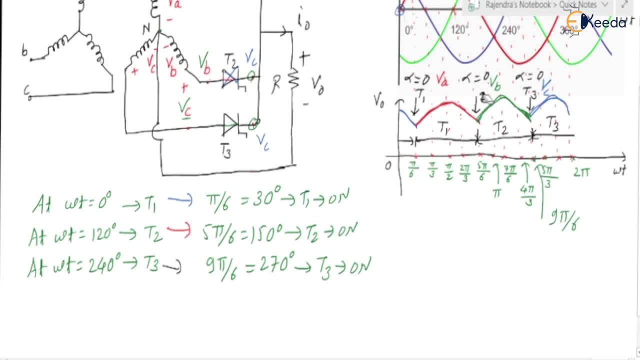 0 for thyristor T3.. Alpha 0 for thyristor T1,. alpha 0 for thyristor T2 and alpha 0 for thyristor T3.. Is this clear? Okay, So this is the waveform of V0 for alpha equal to 0 degree. Is this clear? 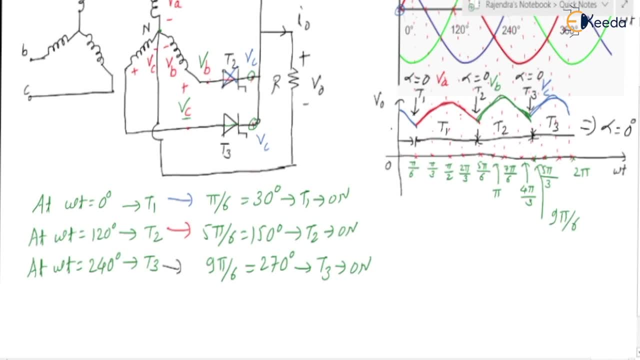 Okay. So if you check here, yes, first of all, the V0 will be same as the top of the VC. Okay, At the starting period. at this instant, VA and VC become same And after that, thyristor T1 turns. 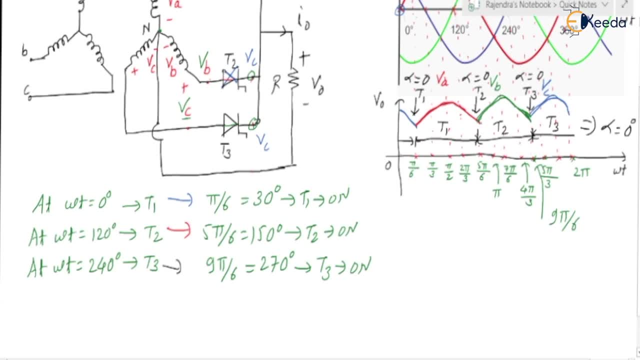 on and output voltage will be VA Right. After that, VA decreases. here And again, VA VB becomes equal. After this instant, that is, 55 by 6, the output will be getting the VB Right And similarly. 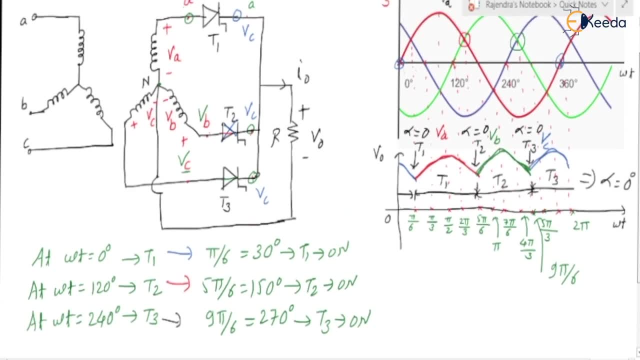 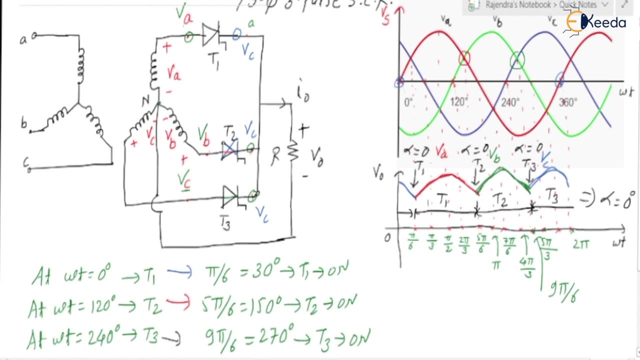 we will be getting the VC Okay. So, if you check, the input is three-phase AC supply. It is having positive values As well as negative values, But output is a DC voltage Right Because it is having only single polarity Right. So that is why it is a DC. Is this clear? Are you getting the point, Okay? So 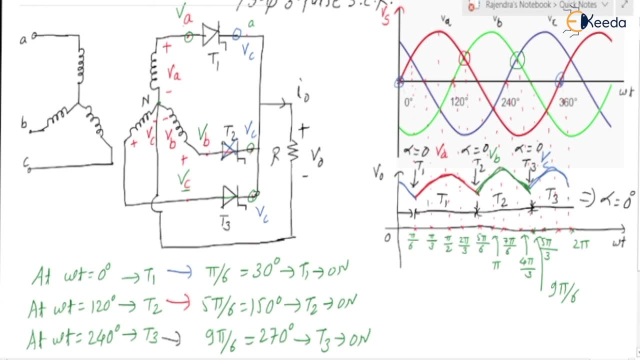 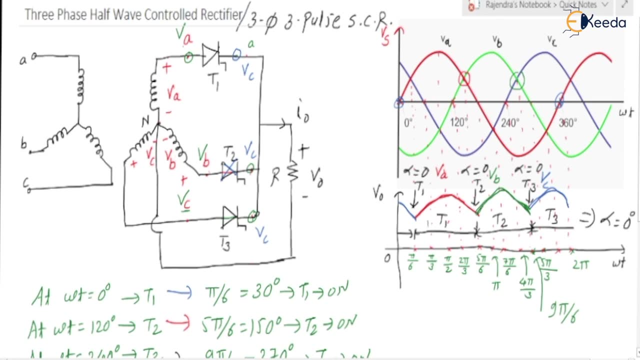 this is the waveform for alpha equal to 0 degree. Okay, Alpha equal to 0 degree, Right. Next, corresponding to one input cycle. corresponding to one input cycle in the output. corresponding to one input cycle in the output. we are getting three pulses: 1, 2, 3.. So that is why it is. 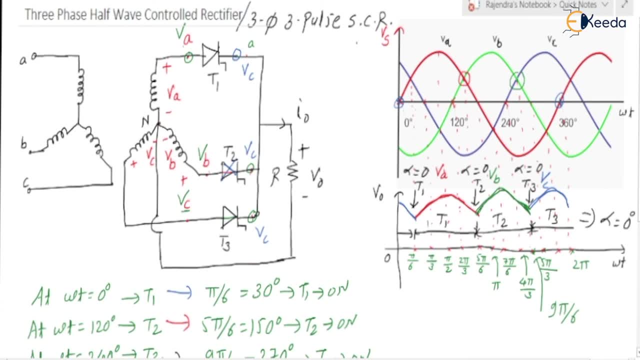 known as the three-phase, three-pulse SCR. Right Three-phase three-pulse SCR. Okay, In the next video we are going to discuss the circuit operation for non-zero value of alpha. For non-zero value of alpha. Thank you. 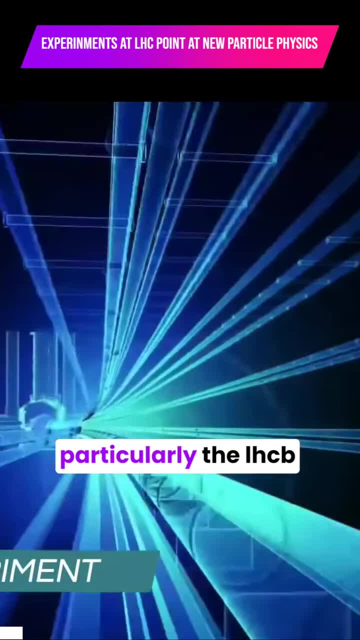 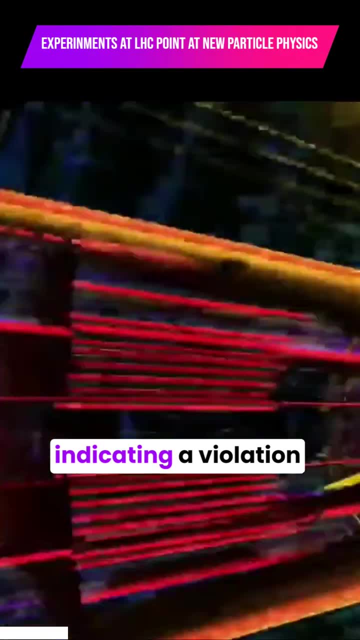 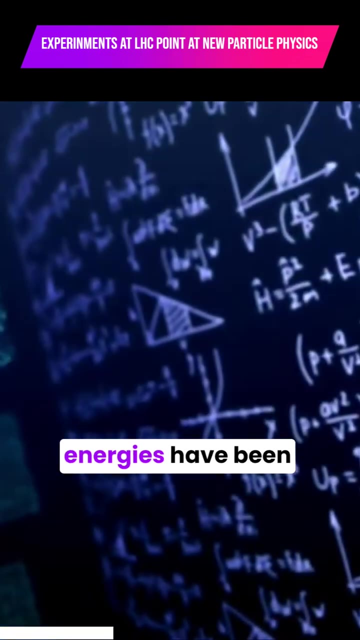 The LHC's experiments, particularly the LHCb experiment, have observed differences in the behavior of particles and their antiparticles, indicating a violation of CP symmetry. Similarly, violations of Lorentz invariance at high energies have been hinted at. 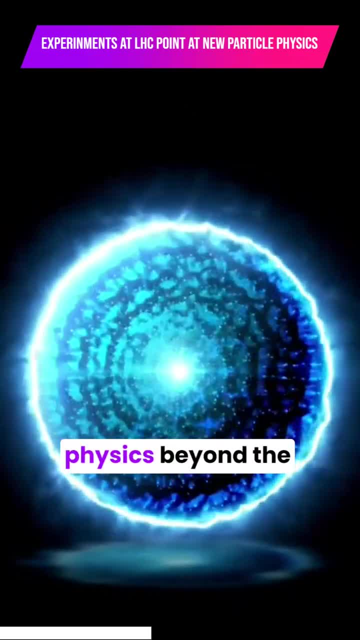 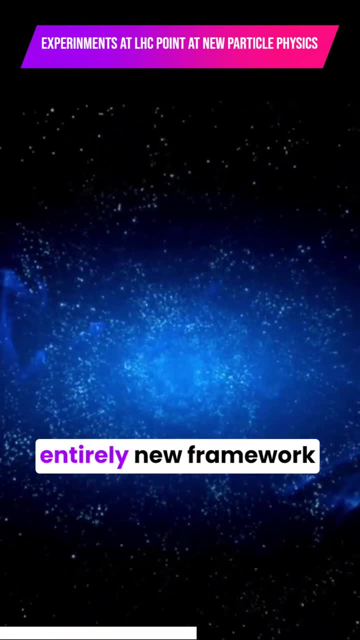 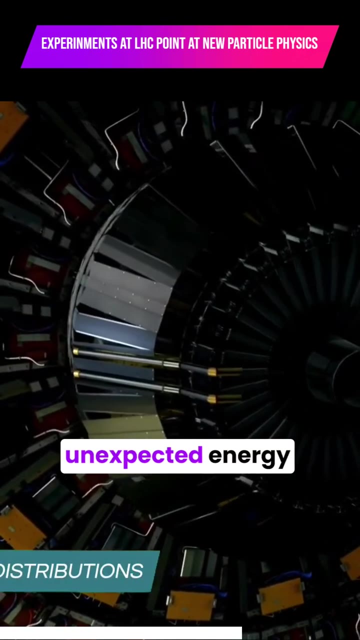 These unexpected asymmetries could point to new physics beyond the standard model, suggesting unknown forces or particles at play, or even a need for an entirely new framework to describe the universe. In addition, the LHC has observed unexpected energy distributions in proton-proton collisions. 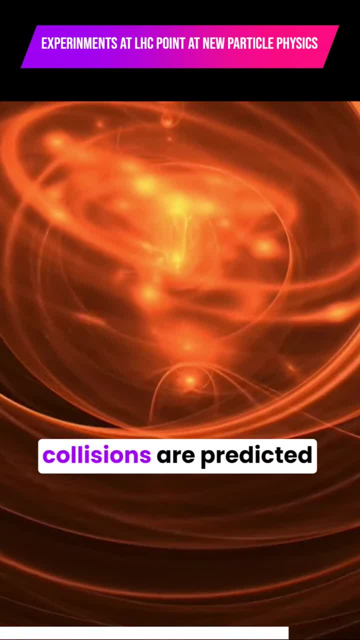 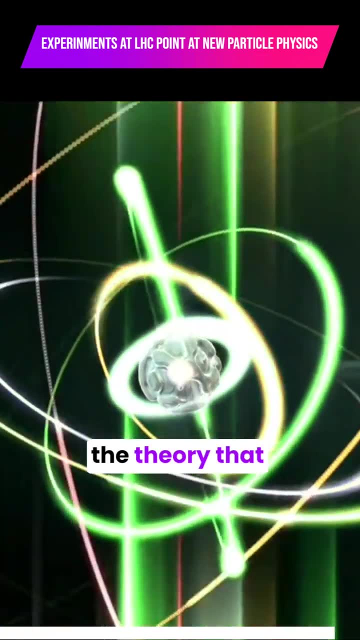 These energy distributions of particles created in collisions are predicted by the standard model based on quantum chromodynamics, or QCD. The theory that describes the strong nuclear force binding quarks to a particle is the theory that describes the strong nuclear force binding quarks to a particle. The theory that describes the strong nuclear force binding quarks to a particle.